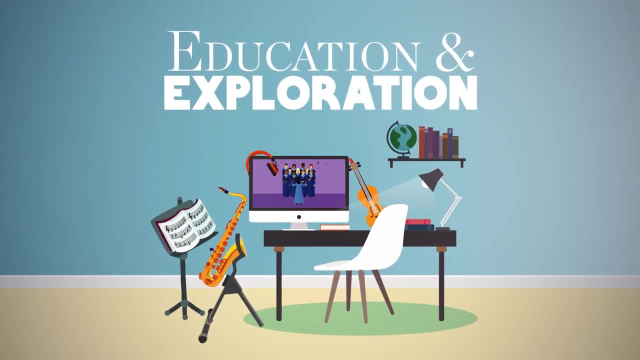 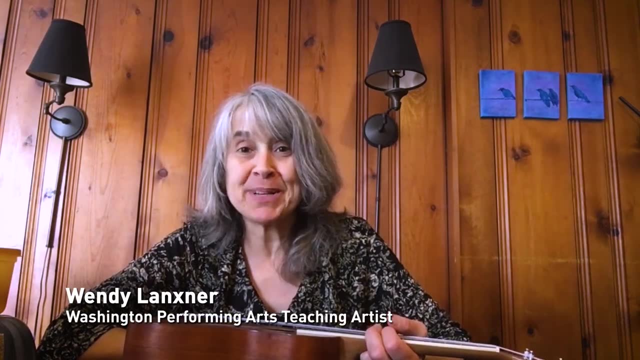 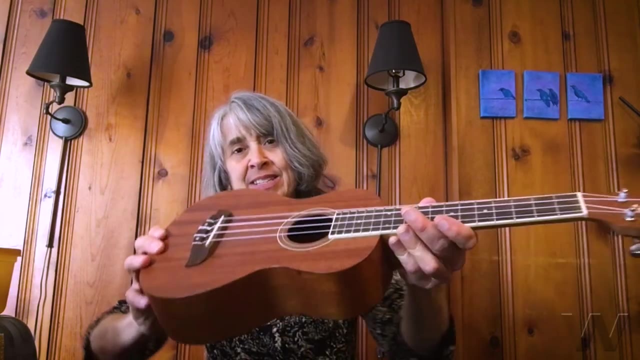 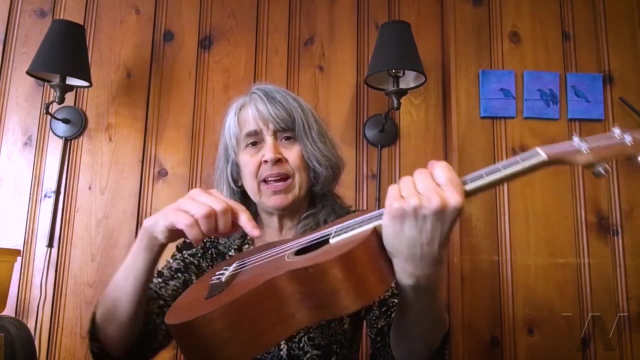 Okay, so let's think about stringed instruments now. How could we make a stringed instrument? I happen to have a ukulele here and you can see it's got strings, obviously, And this part of the ukulele is a resonator, so it allows the sound from the string to be amplified. 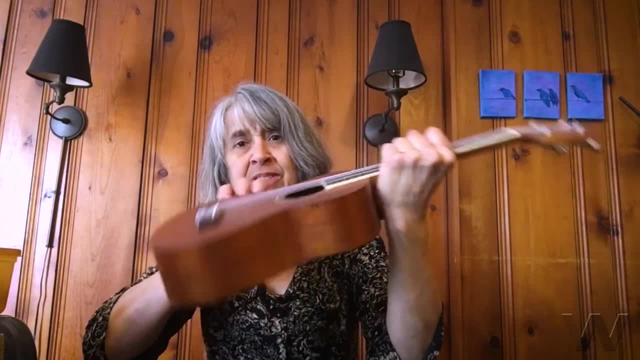 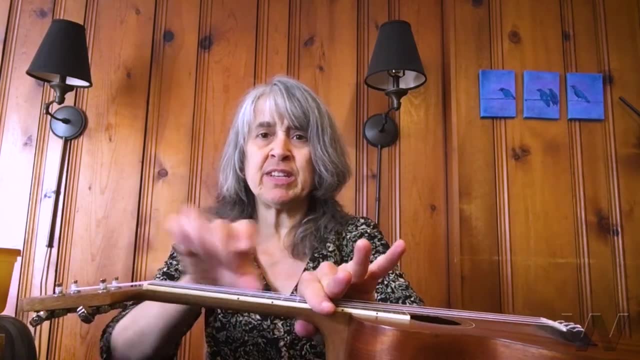 so you can hear it. You can imagine, if you didn't have this part, and you only had this part, it wouldn't make too much sound. In fact, let me just try something, So I'm going to stop the strings here and just pluck them here. See, it doesn't really sound very good. 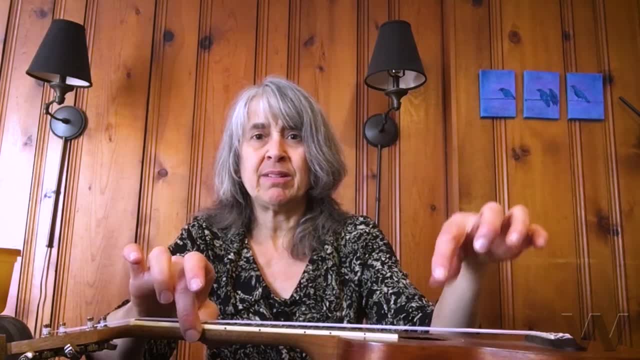 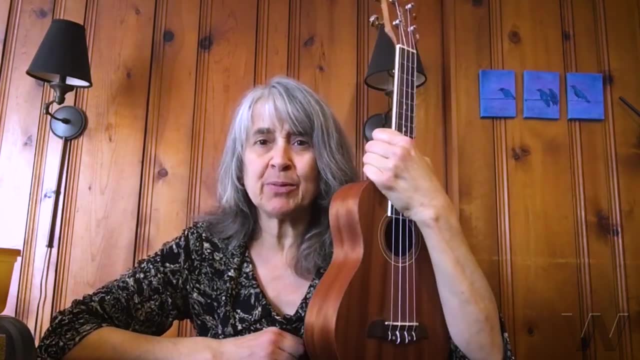 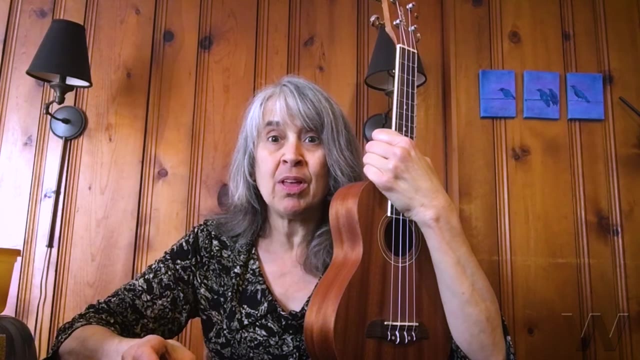 Whereas if you let the whole string vibrate, you can hear it better because it's resonating here. I don't know if you've ever tried this, but like with a music box, if you hold it up You can hear the sound, but if you put it on the table, suddenly the sound is bigger. 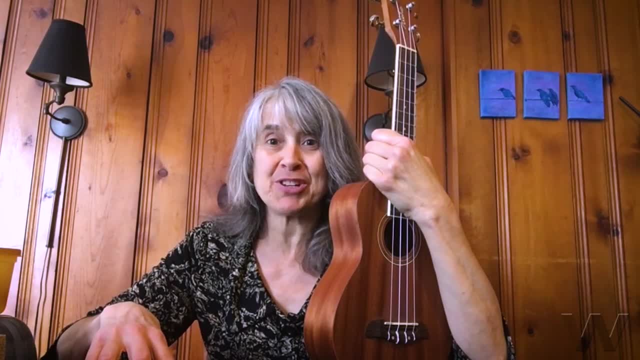 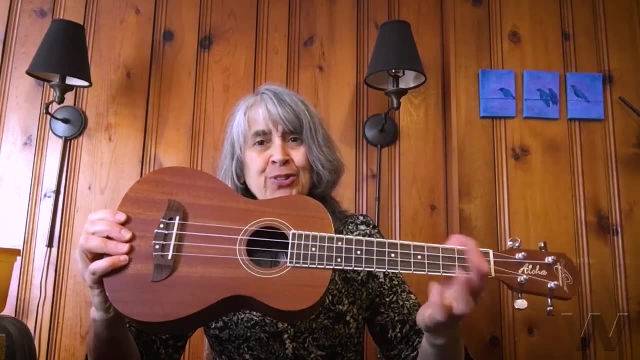 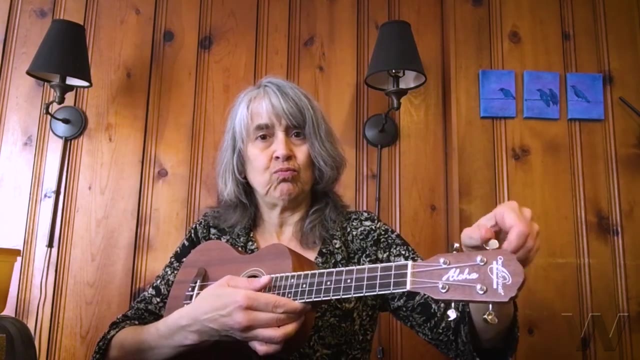 because the table is amplifying the sound vibration. So what we need is some kind of box and a string stretched kind of tight. If the strings are loose they're not going to make much sound. In fact, I'm going to take this ukulele here, I'm just loosening. 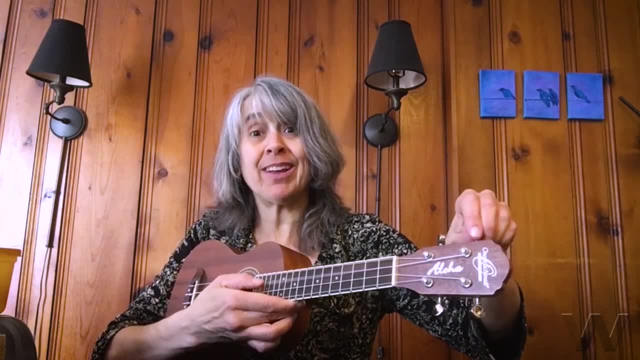 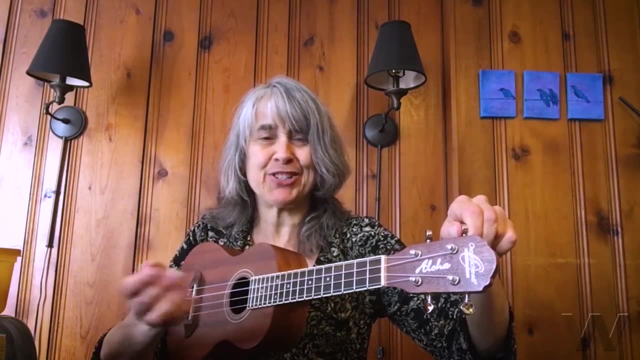 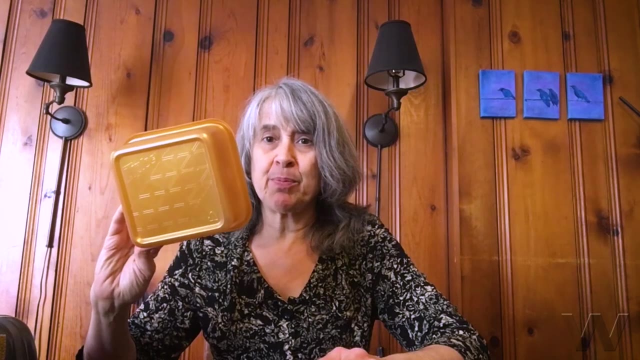 one of the strings. So the tighter the string, the higher the pitch, right Yeah, when it's really loose it just kind of doesn't sound like much. So let's see what we can find. Okay, I found this box, this plastic kind of Tupperware box, and some rubber. 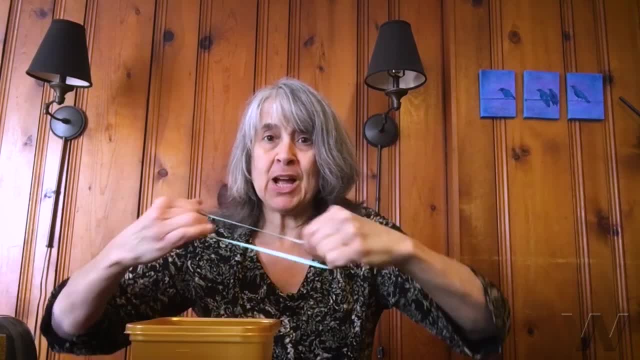 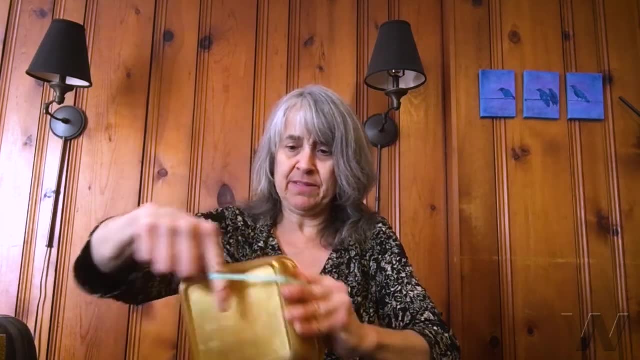 bands which I thought, well, I could probably stretch them pretty tight. I hope they don't break. I don't have too many, So I'm just going to stretch it around this box here and see if it makes a sound. I'm going to try a couple of them. 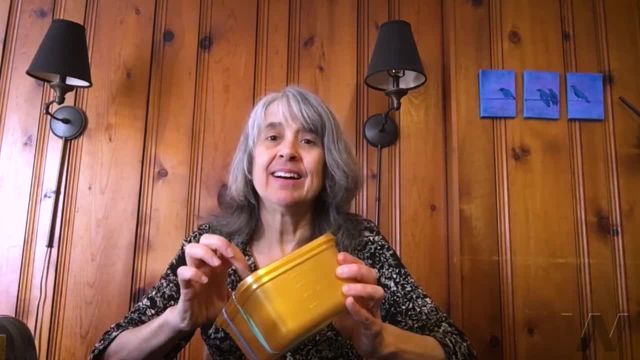 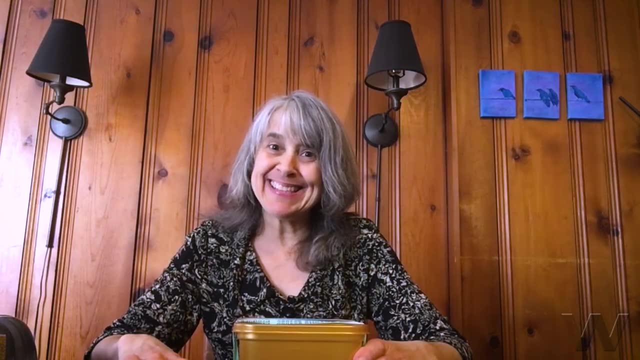 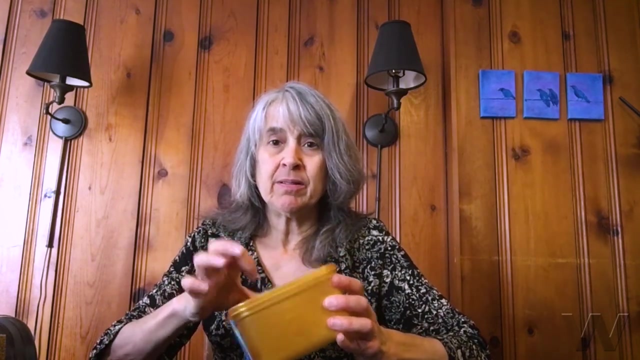 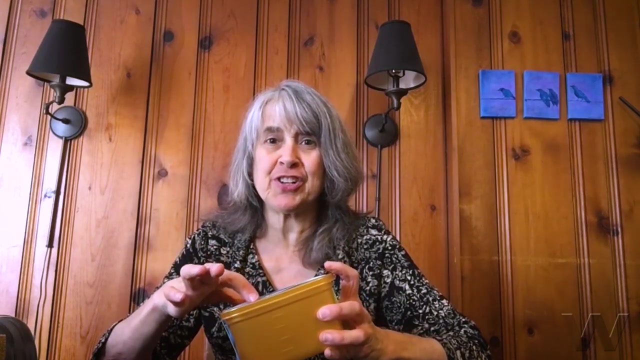 Oh my gosh, amazing. Oh wow, look what I just discovered. So I put three rubber bands on here and this one. if I pull, if I leave this side where it is and just pull here and kind of redistribute how it's stretched, that's the same rubber band. I loosen it. 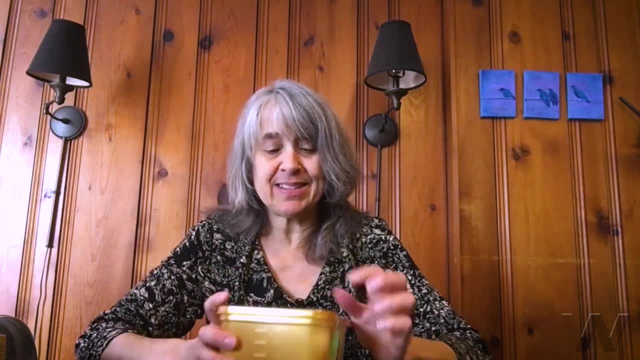 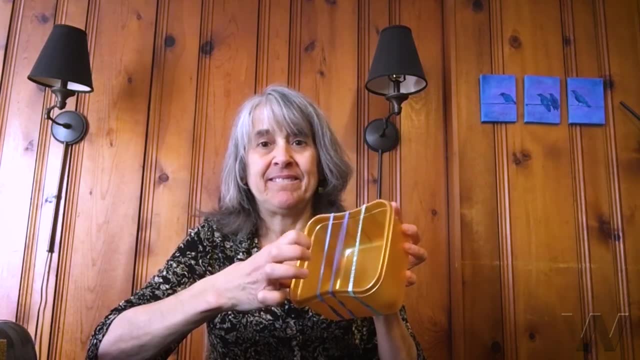 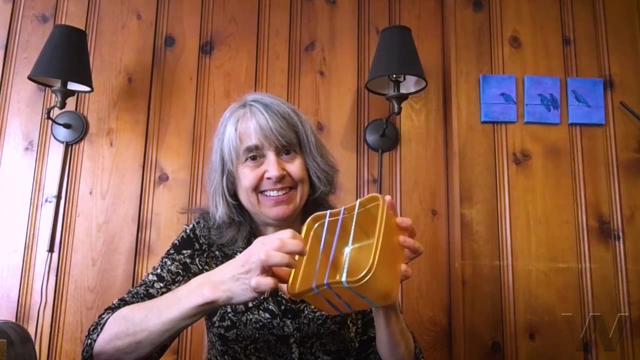 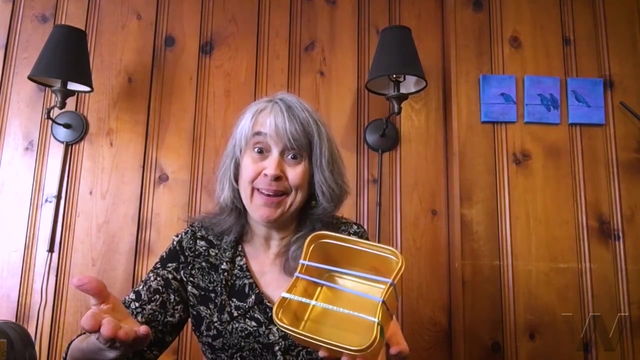 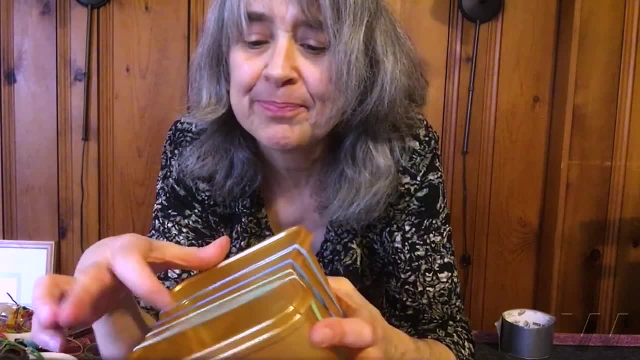 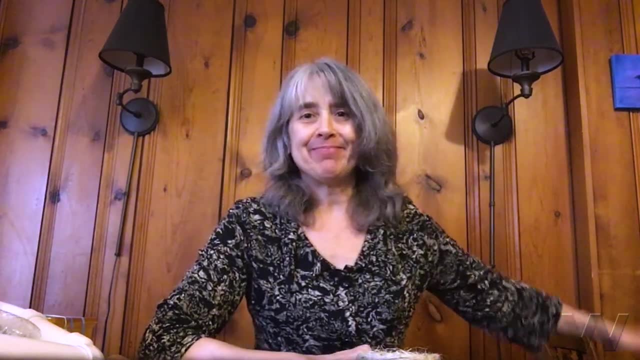 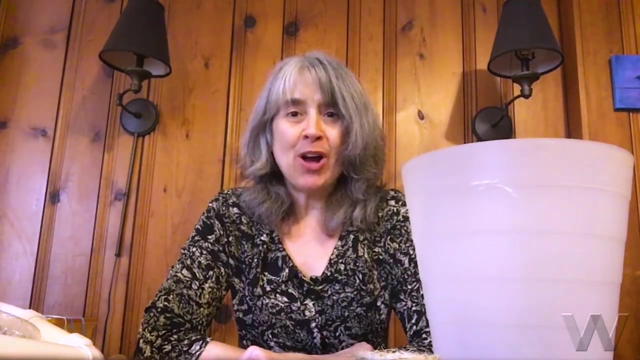 That's better. All right, guys, now I'm feeling kind of ambitious. So I have this trash can, and I don't know if you've ever heard of a washtub bass, but it was a bass guitar people used to make. 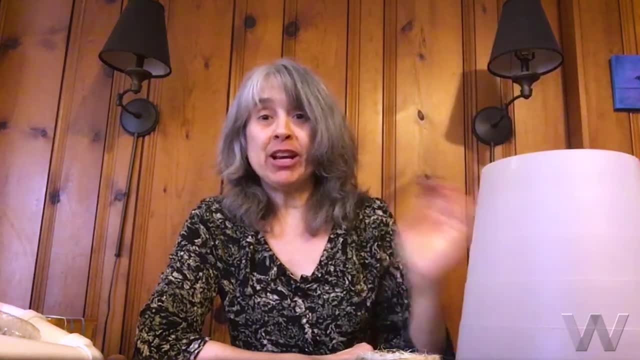 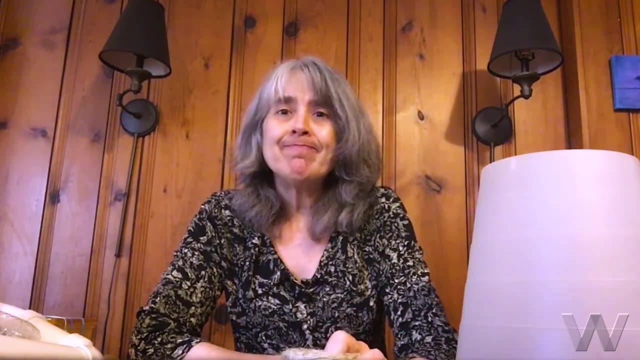 Well, they probably still do. Made out of a trash can, some string and some sort of long stick, It was like a handle off a broom. Anyway, I'm game, Let's give it a whirl. I have two words to say right now. Parental consent. 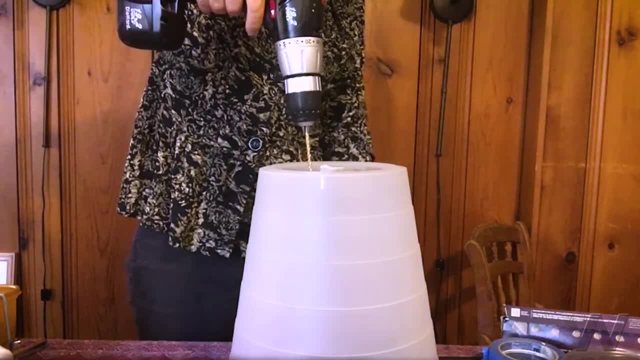 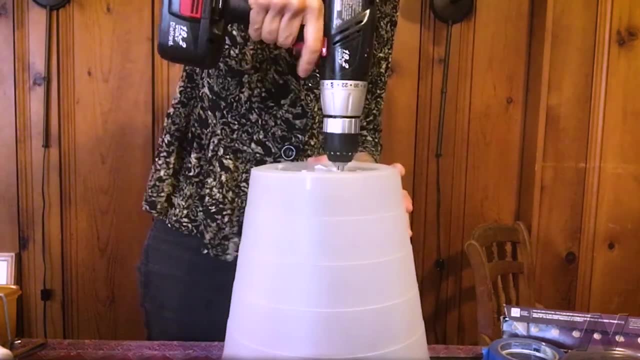 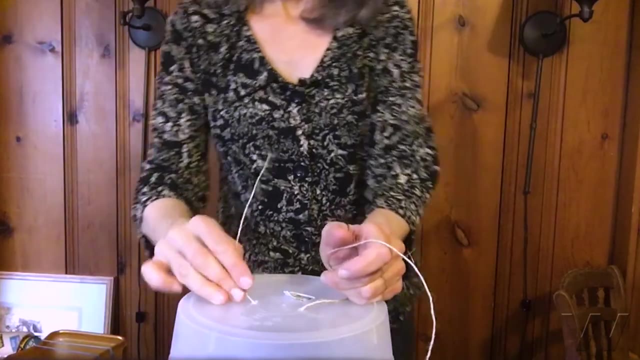 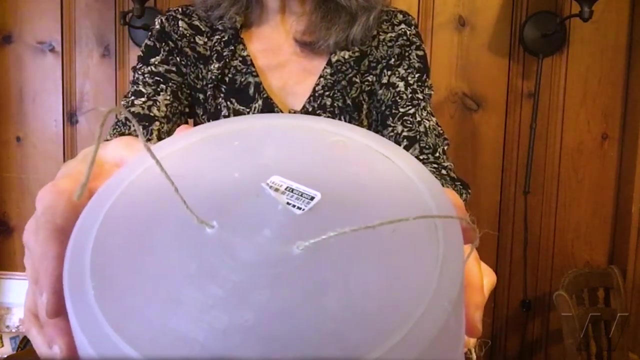 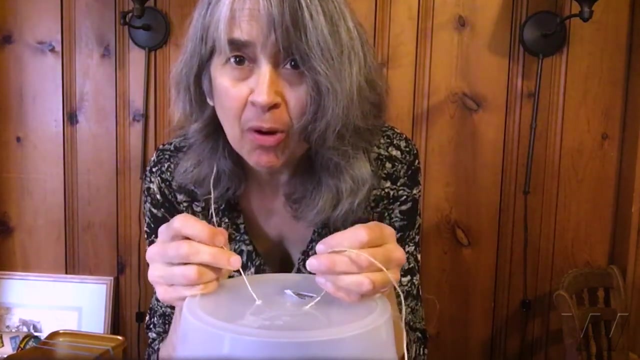 I love power tools. I cut a really long piece of twine and I threaded it through the two holes like that, and I'm going to attach it with a square knot. This is a really good knot to use if you don't want something to come apart. 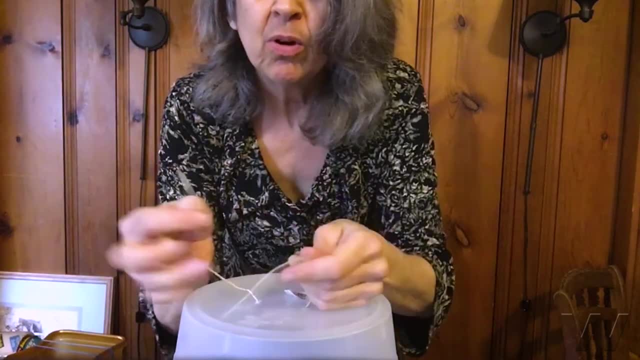 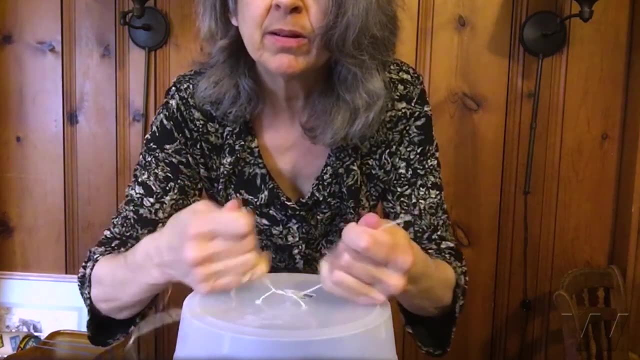 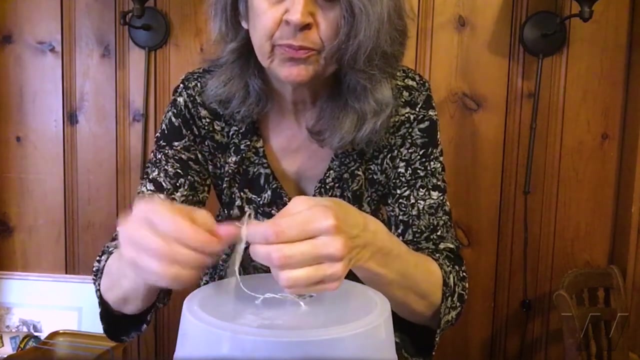 So you take one side and you go over the other one. So I'm going right over left and then put it through as usual: right, Pull it tight. Now I'm taking that side, which is now on this one, And I'm going over the other one and through. 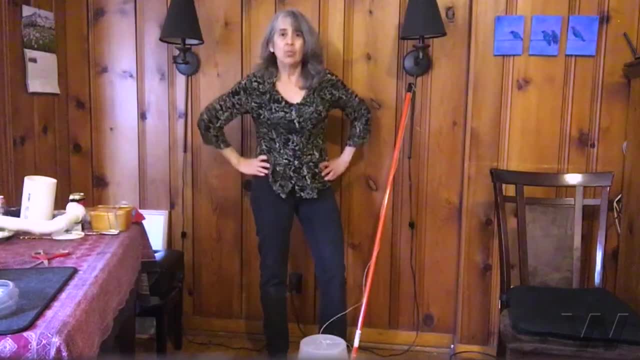 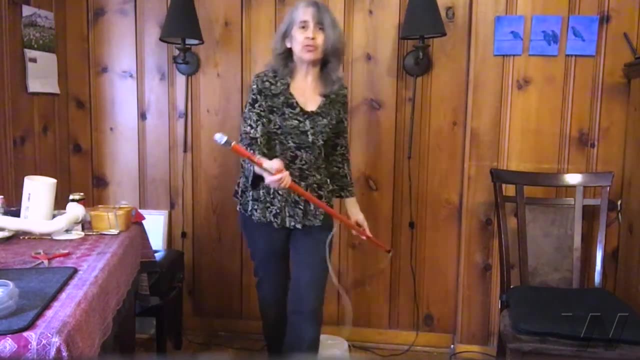 Boom, That is not going to come off. Well, I totally lucked out. I have this handle that you can attach a paint roller to in my closet. Get out of there, Come on. come on, come on, Okay, ready, Check this out.